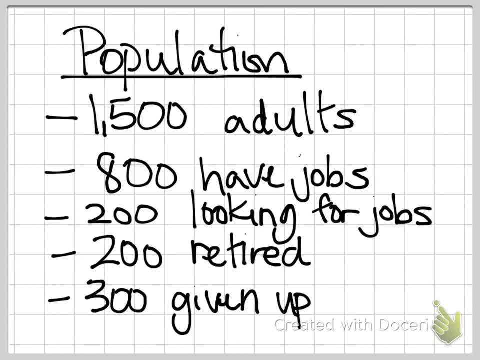 Here's the example that we're going to work through. We have a hypothetical country. It has 1,500 adults, 800 have jobs, 200 are looking for jobs, 200 are retired and 300 have given up looking. 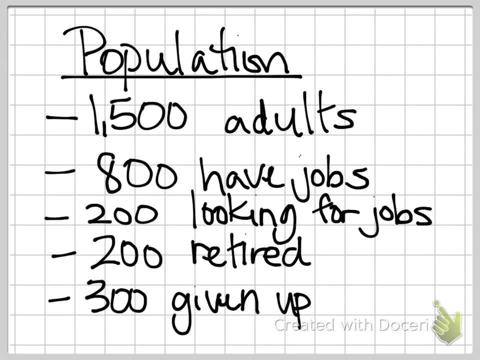 They aren't working, They're not applying for anything, They're just kind of sitting at home. This group, these are not unemployed people. We call them discouraged. We call them discouraged workers. They are not in the statistics that we run. We're not even going to consider them in our calculations. 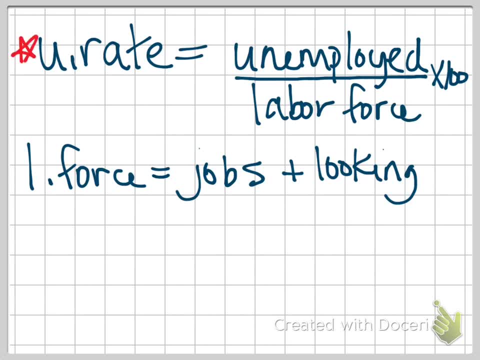 Here is an important formula that you need to calculate these: our unemployment rate formula. Our unemployment rate is calculated by taking the number of unemployed and dividing that by the labor force and then multiplying times 100.. Remember, our labor force is comprised of two groups of people: the people that have jobs currently, both full-time and part-time- and the people that are actively seeking jobs. 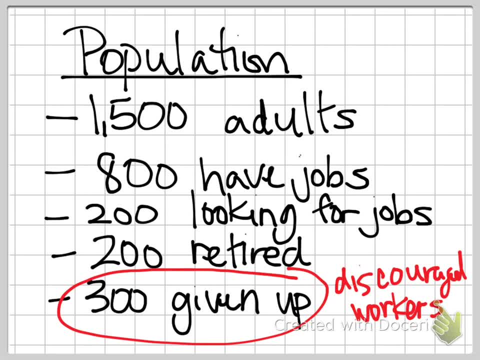 If we go back here, we would see that we have 800 people that have jobs and we have 200 people that are looking for jobs. This 200 here, these are the only ones. These are the only ones that, in our economy right now, we would say are unemployed. okay. 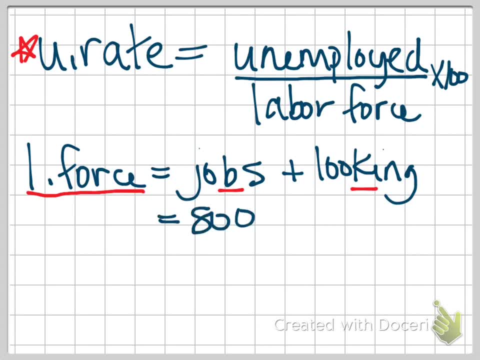 So our labor force is going to be the 800 plus the 200 who are looking, or 1,000 people. So again to calculate then the unemployment rate, we're going to take those 200 who are unemployed, divide by that full labor force number of 1,000, and then multiply that. 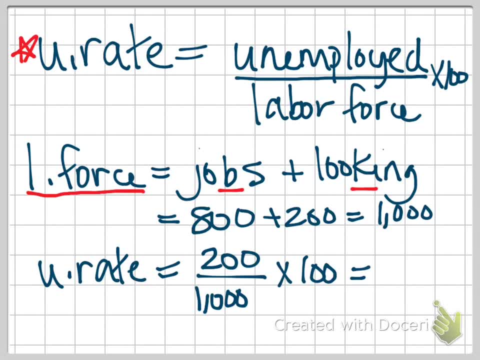 You end up with 300 times 100. So if you do this calculation out, you would see that this economy has an unemployment rate of 20 percent. So that's really high. okay, The worst ours was- since we've tracked this- was 25 percent at the height of the Great Depression. 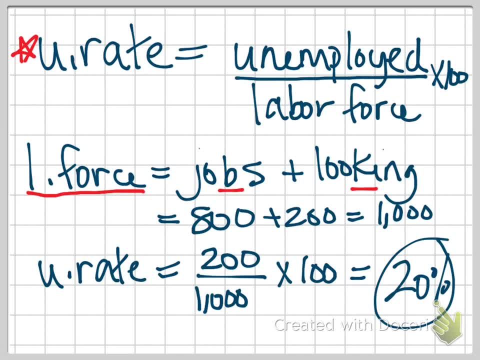 So this would be a very, very high unemployment rate. A couple of things here. Again, you're unemployed. This top number is just These who are actively seeking jobs. Again, you're unemployed. This top number is just tHose who are actively seeking jobs, or the number that you're looking for. This top number that you're looking for is just those who are actively seeking jobs. 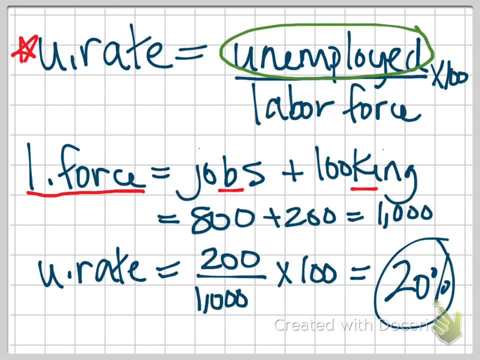 jobs. They're not working but they really want to. They have to be looking to be part of this number. okay, And make sure when you divide, that you're dividing by the entire labor force, those who are working plus those who are unemployed. okay, That 1,000 figure in this example A lot. 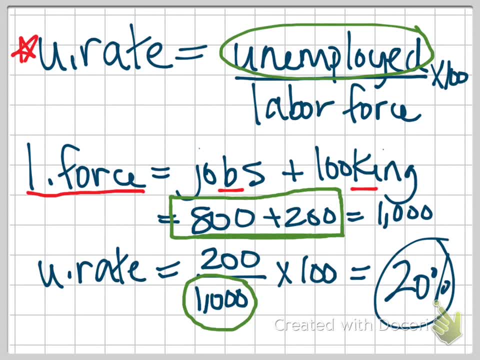 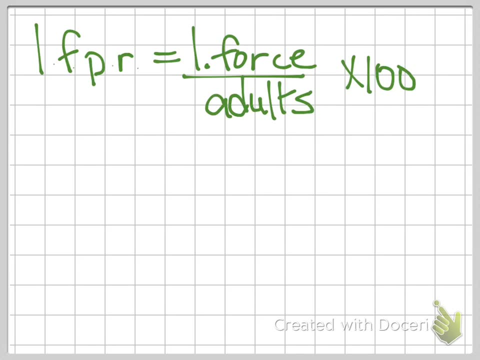 of times, students will just divide by the people that have jobs, the 800, and that will give you the wrong answer. So make sure it's the full labor force. Okay, so now we're going to calculate the labor force participation rate. And so now it's the number in the labor force which we just found. 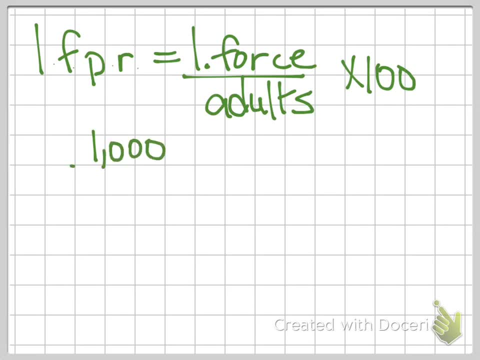 on the previous screen to be 1,000 people. We're going to divide that by all the adults. In this case, I gave you the number. If you were given a total population, you would just need to subtract out the children. okay, to get your total adults. 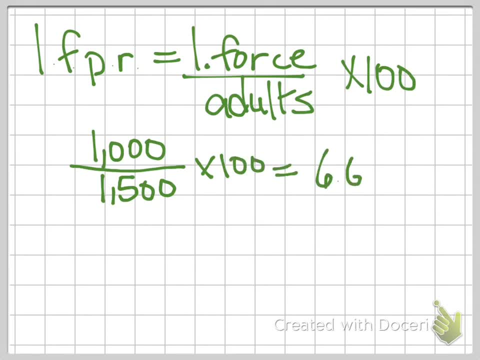 And then we'll multiply again times 100.. If you did the calculation, it is, I messed it up there, I went too fast. 66.67 percent, okay, is our labor force participation rate, And so what this one is. 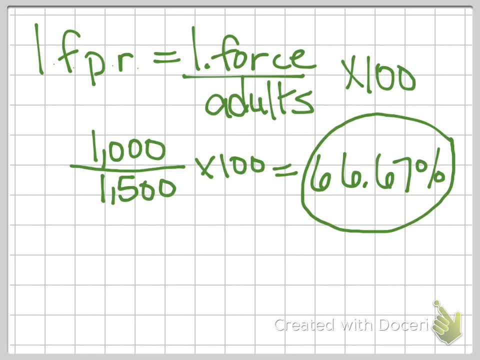 telling us is, of all the adults in our economy, how many of them are either contributing to production or would like to be right? Because, again, the labor force participation rate is the number of adults in the labor force, and that number of adults in the labor force includes both those who are working and those who would like to work. okay, And so what we'll see is that in an economy, let's say, where we suddenly have a lot more people who retire- okay, so, like our baby boomer generation, a big part of our population is starting to retire. So if retirees, if that number goes up, then it's going to cause our labor force participation number to go down. Likewise, if we have 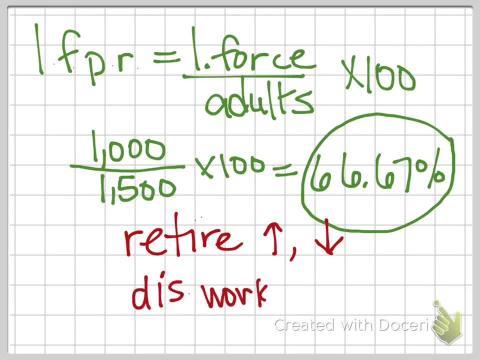 a lot of those discouraged workers, the people that have given up. So if we see the number of discouraged workers increase, then again we'll see our labor force participation rate decrease. The trend that we've seen the past few decades in the United States is that the labor force participation rate for men has decreased. More of them are retiring earlier in their lives, while we've seen more women enter the workforce, So we've seen an increase um the labor force participation rate for our females. 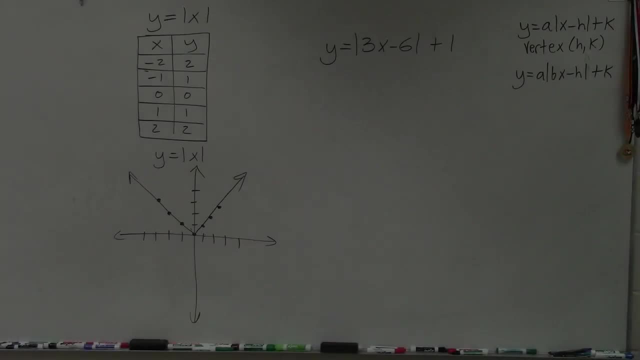 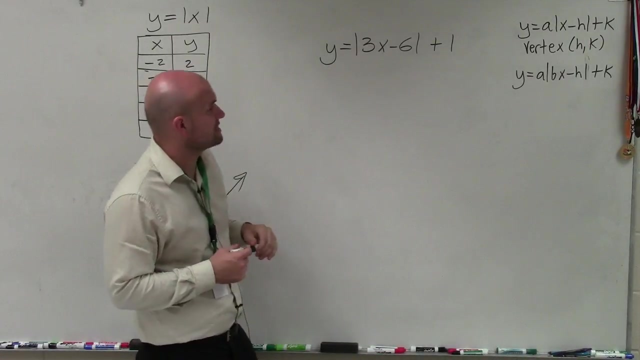 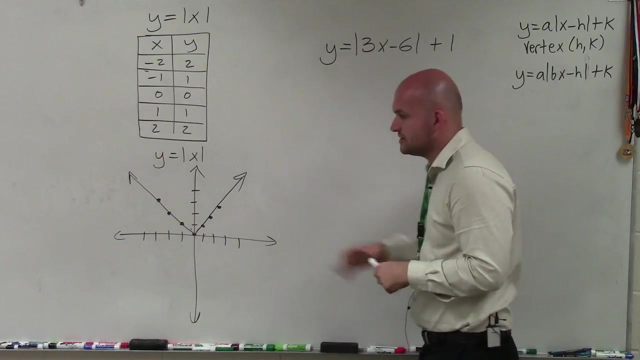 Welcome, ladies and gentlemen. So what I'd like to do is show you how to graph this absolute value equation, which is: y equals absolute value of 3x minus 6 plus 1.. So to graph an absolute value equation, the first thing to do- is very important- is to understand what 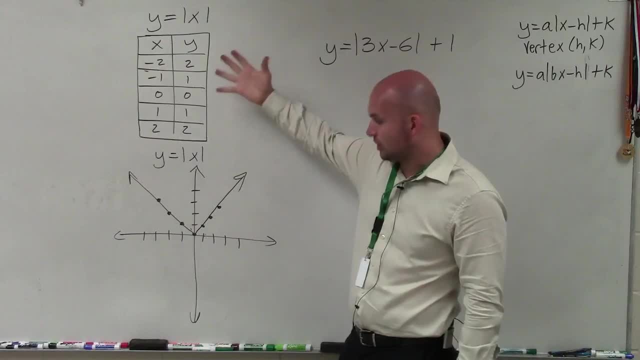 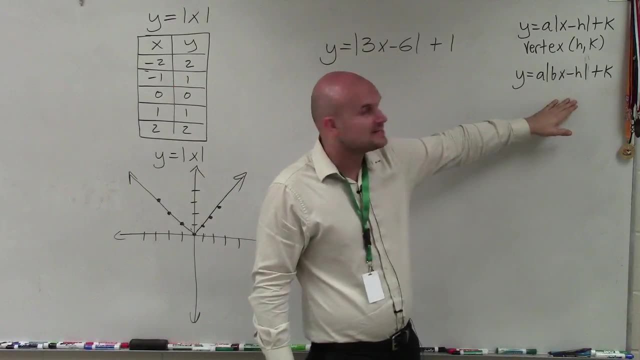 does exactly the absolute value equation look like, as well as the table, and then what are they going to be in our new transformation? So you can see, here we have this 3x minus 6. So it's going to look something like this. So I can't just say that my vertex is going. 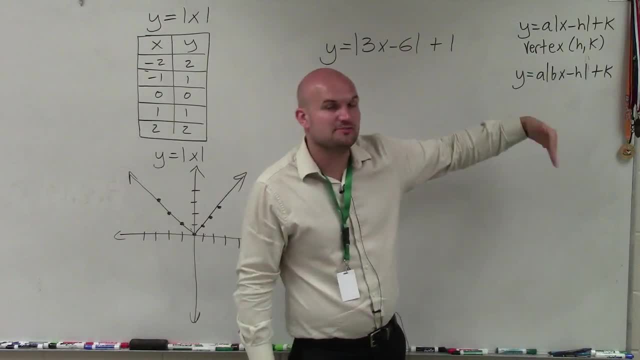 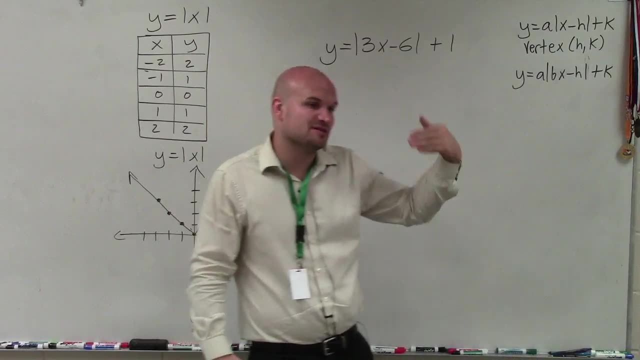 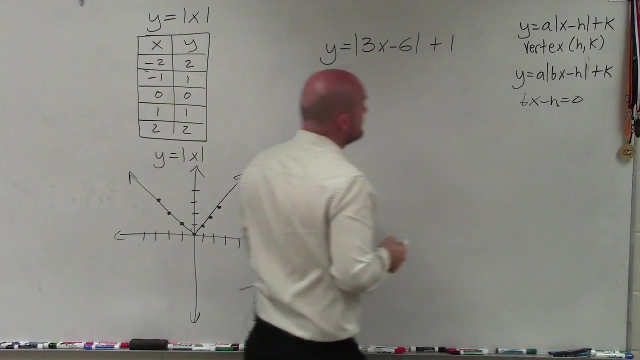 to be hk, because this b is actually going to be affecting my vertex. However, my graph is shifting up one That is going to be my new k value of my vertex. But to find the new x value, what I simply need to do is take my bx minus h and set it equal to 0.. And that's. 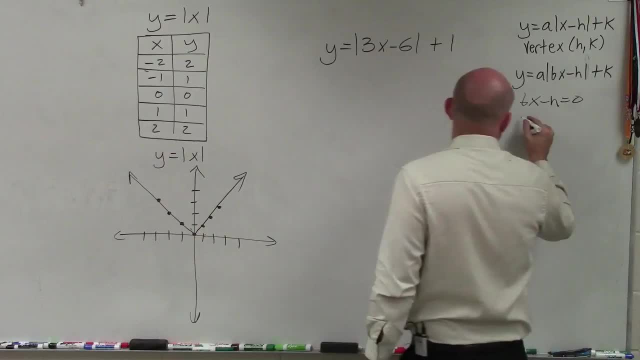 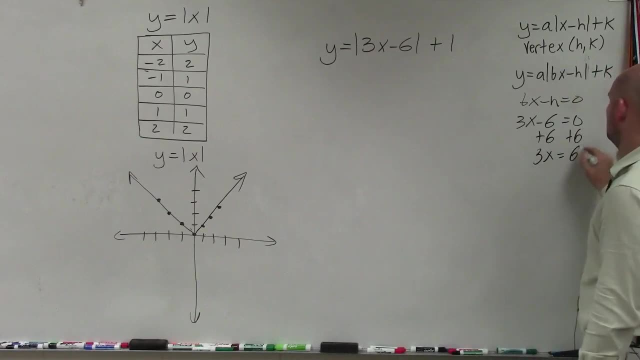 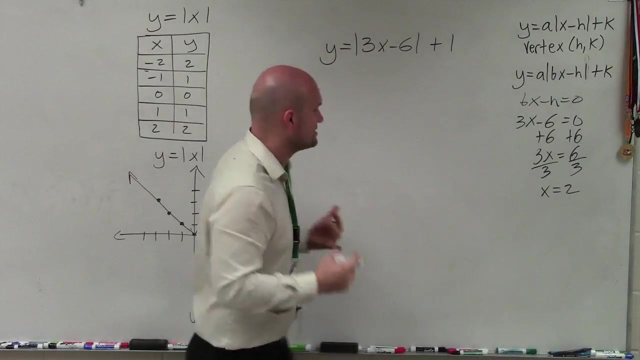 going to be the new x value of my vertex. So to do that, I simply just take 3x minus 6, set it equal to 0. Then I solve for x: x equals 2.. Now that is my new x coordinate of my vertex. So my 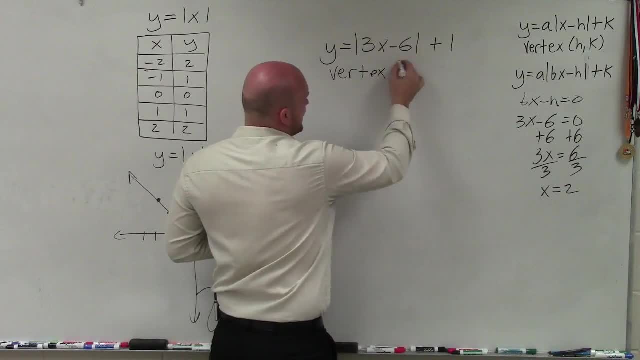 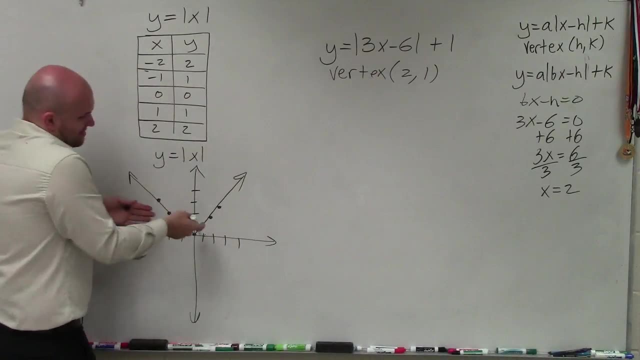 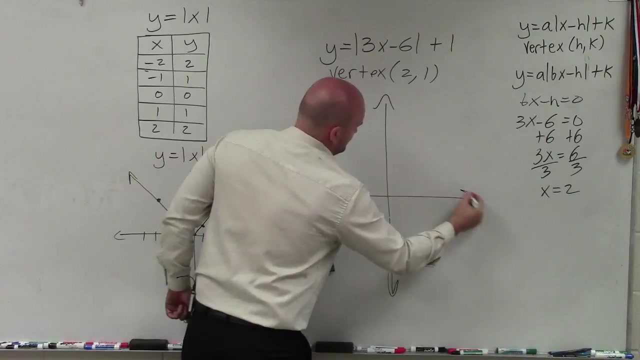 vertex is not going to be at 6, but now my vertex is going to be at 2 comma 1, where 1 is still going to be my k, which is going to be represented. So, basically, what I'm doing is I'm taking this graph and I'm shifting over two units and one unit up, One, two. 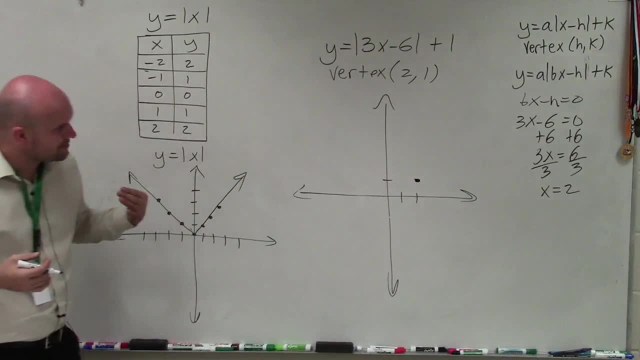 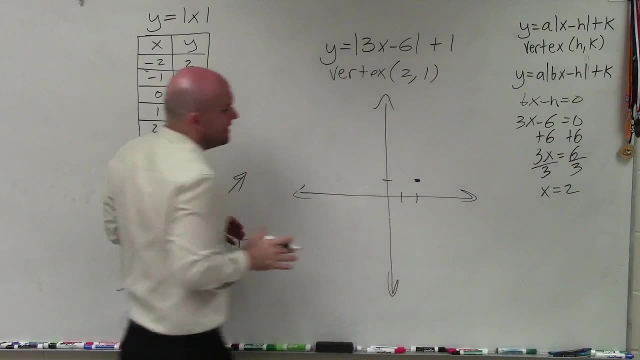 up one unit Now. the next thing I want to do is I need to be able to identify what exactly is my graph going to look like, And I can't take this graph and just plug it in there, because this b is what the b is going to be doing, That's going to now vertically stretch.